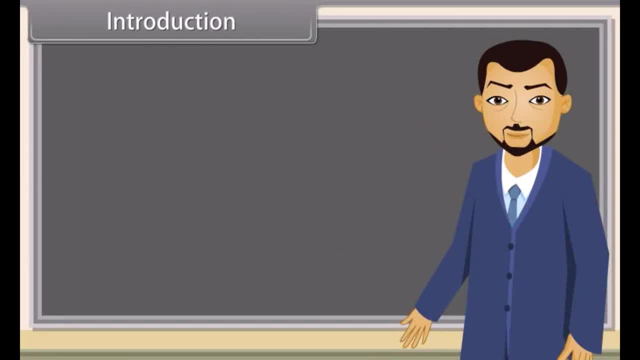 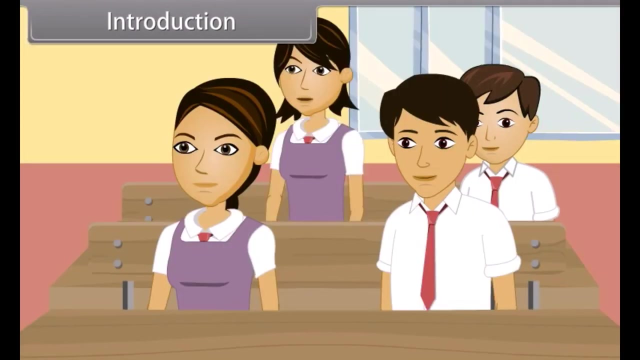 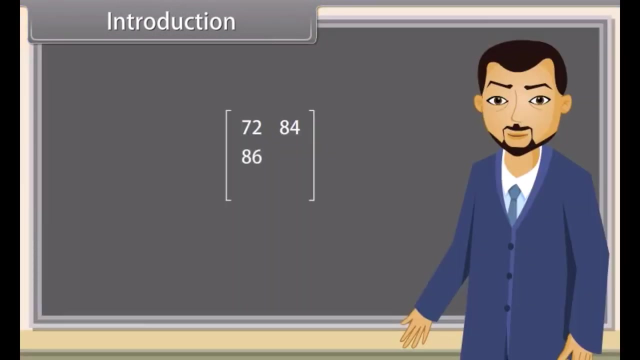 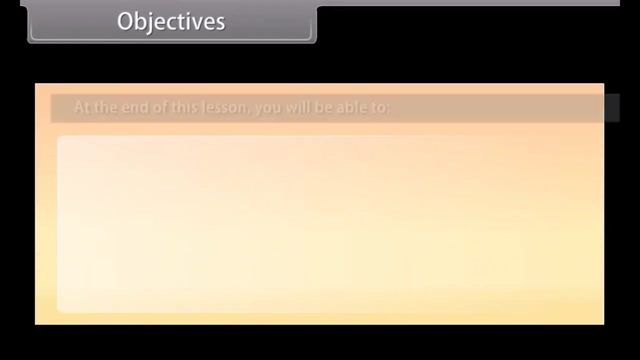 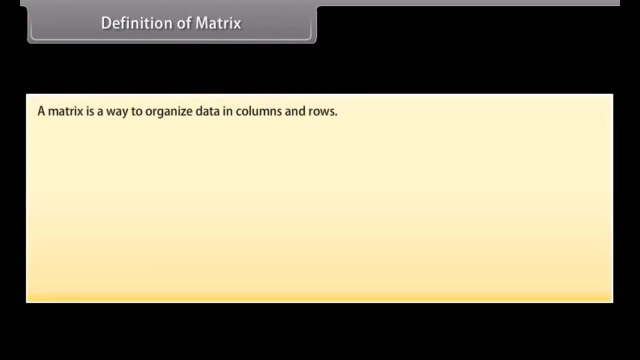 Introduction. Introduction: Come, let's start Objectives: At the end of this lesson, you will be able to Define matrix, Explain order of matrices, Write different types of matrices. Define zero matrix. Understand equality of matrices. Understand addition of matrices. Definition of matrix: A matrix is a way to organize data in columns and rows. 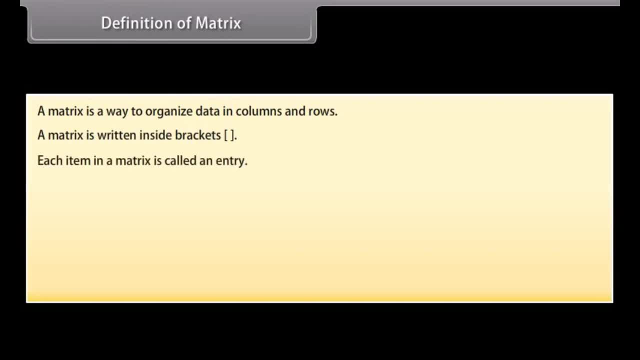 A matrix is written inside brackets. Each item in a matrix is called an entry. Look at this matrix. It has two rows and three columns. The entries of the matrix below are 2, minus 5, 10, minus 4, 19, 4. 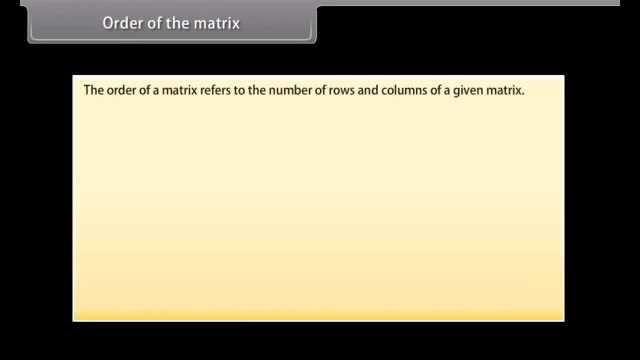 Order of the matrix. The order of a matrix refers to the number of rows and columns of a given matrix. By convention, the order of a matrix is given by number of rows, by number of columns. Here we can see two pictures of the same matrix. 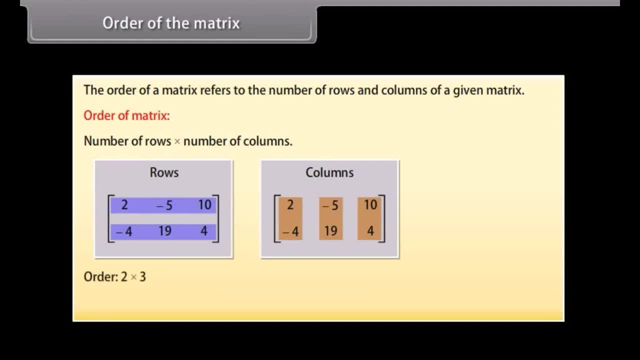 with the rows and columns highlighted. The order of this matrix is 2 by 3, that is, 2 rows by 3 columns. The order of the matrix refers to the number of rows and columns of a given matrix. The order of the matrix refers to the number of rows and columns of a given matrix. 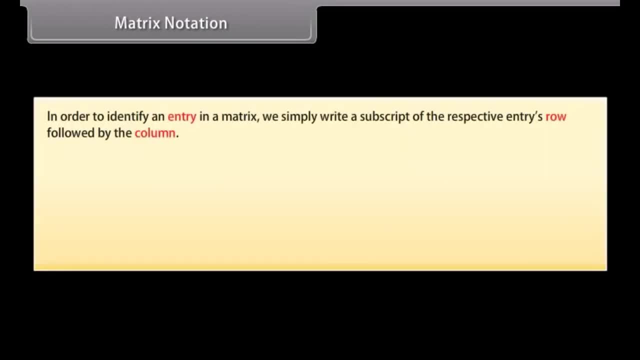 Matrix notation. In order to identify an entry in a matrix, we simply write a subscript of the respective entries row, followed by the column. In matrix A, we write A23, to denote the entry in the second row, and the third column, A23, indicates the row number 2 and the column number 3.. 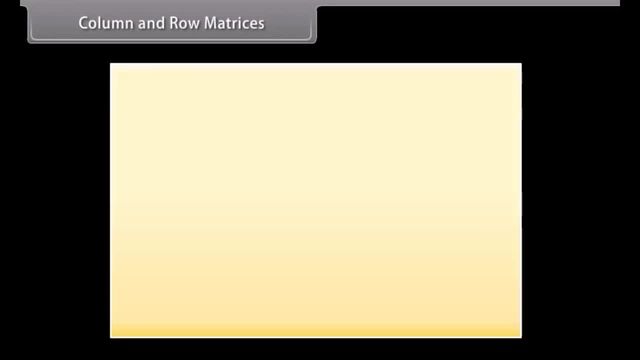 Column and row matrices. Column matrix: A matrix which has only one column is called a column matrix. Example of column matrix: A is equal to column wise, 21,, 17,, 9.. This matrix has three rows but only one column, So it is a column matrix. 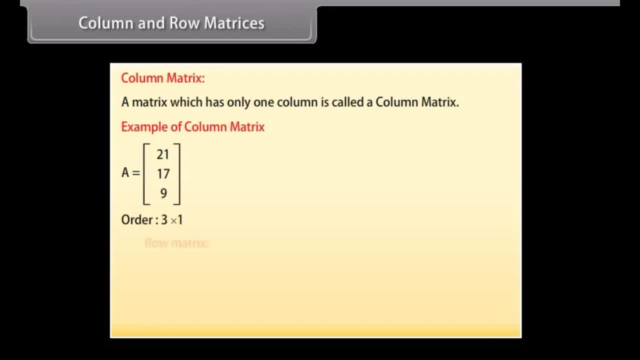 Its order is 3 by 1.. Row matrix: A matrix is said to be a row matrix if it has only one row. For example, row wise 3,, 5, 1 is a row matrix as it has only one row. 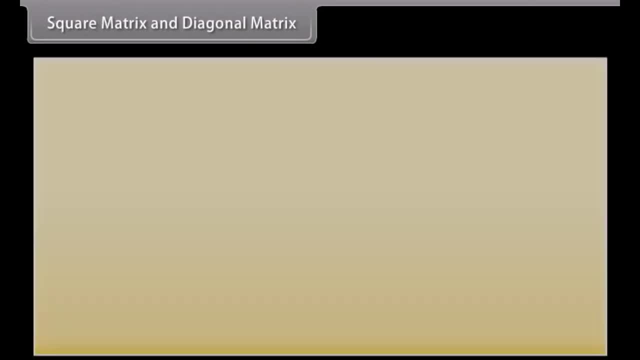 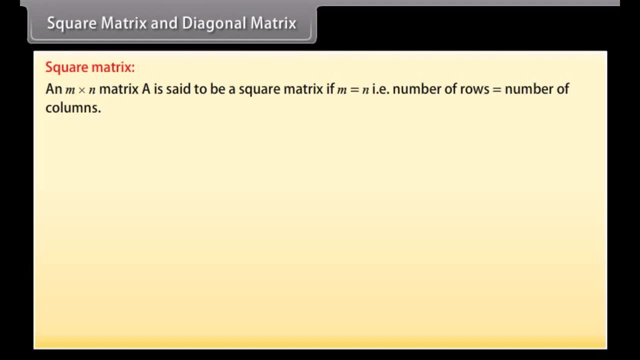 Square matrix and diagonal matrix. Square matrix and diagonal matrix. Square matrix: An M by N. matrix A is said to be a square matrix if M is equal to N, that is, number of rows is equal to number of columns. For example, A is a square matrix of order 3 by 3.. 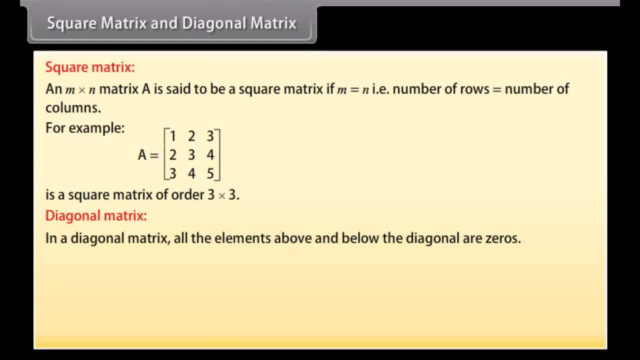 Diagonal matrix. In a diagonal matrix, all the elements above and below the diagonal are zeros. For example, B is a diagonal matrix or an array of three rows. It is actually called R, math Symbolically N. anduar is symmetric, readable physical form. 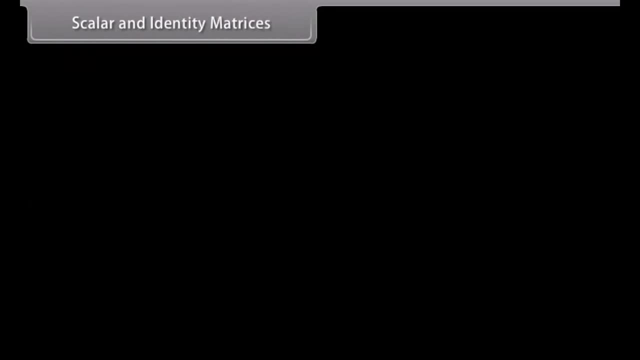 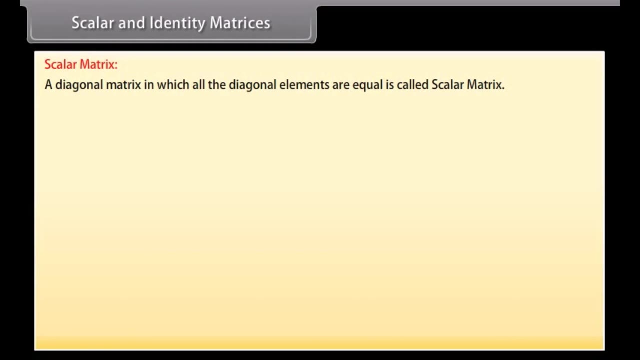 funktionally correct. Scalar and identity matrix. Scalar matrix- A diagonal matrix in which all the diagonal elements are equal is called scalar matrix. Look at this matrix. It is the diagonal matrix with the diagonal elements same, that is seven. Therefore it is a scalar matrix. 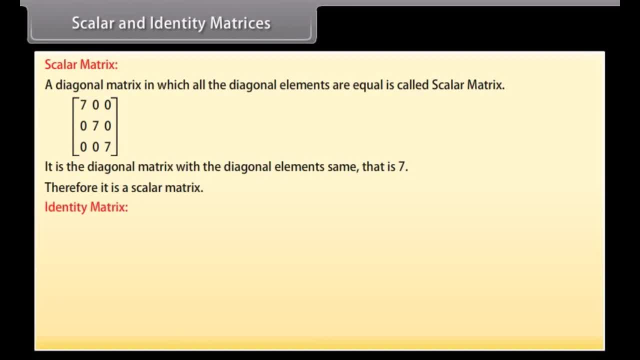 Agnel matrix is aussen после other diagonal elements equal ol, that is 7. Identity Matrix: A square matrix in which all the main diagonal elements are 1s and all the remaining elements are 0s is called an Identity Matrix. 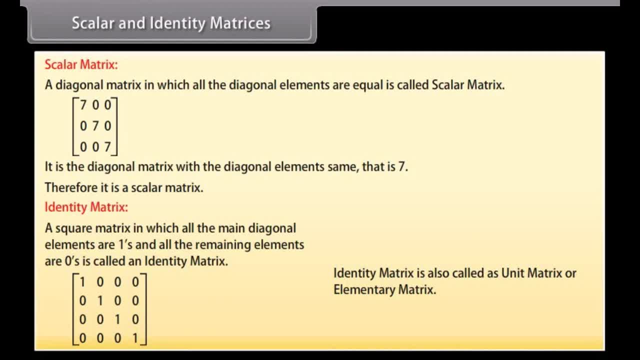 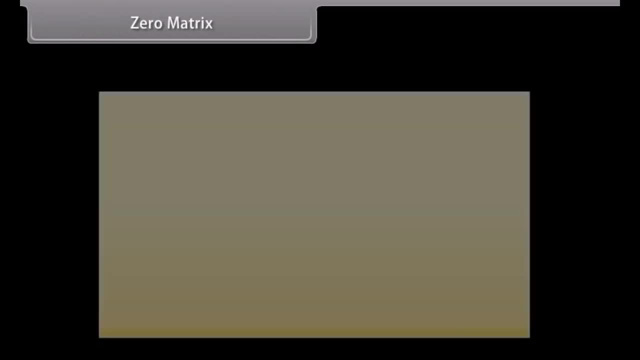 Identity Matrix is also called as Unit Matrix or Elementary Matrix. Identity Matrix is denoted with the letter n by n, where n by n represents the order of the matrix. Zero Matrix, A zero matrix or null matrix is one which has all its elements 0.. 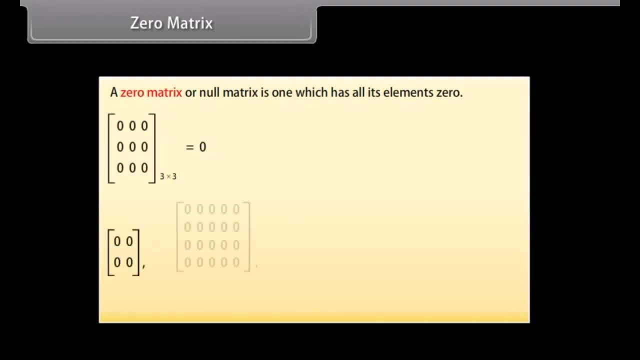 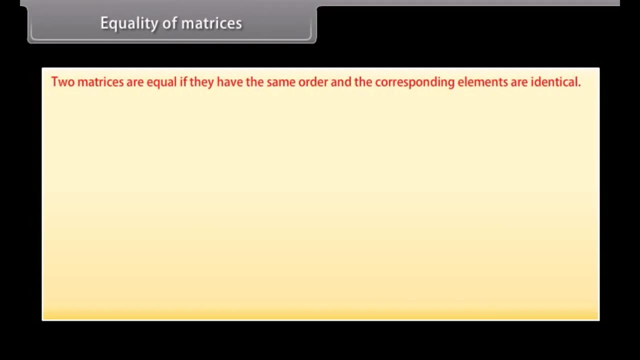 Here is a 3 by 3 zero matrix. These are three more examples of zero matrix. The zero matrix is denoted by 0.. Equality of Matrices. Two matrices are equal if they have the same order and the corresponding elements are identical. 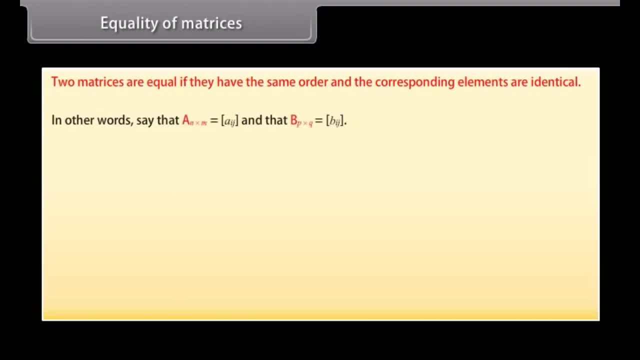 In order. other words, say that a- n by m is equal to a i j and that b- p by q is equal to b i j. then a is equal to b if, and only if, n is equal to p, m is equal to q and a i j is equal to b i j. 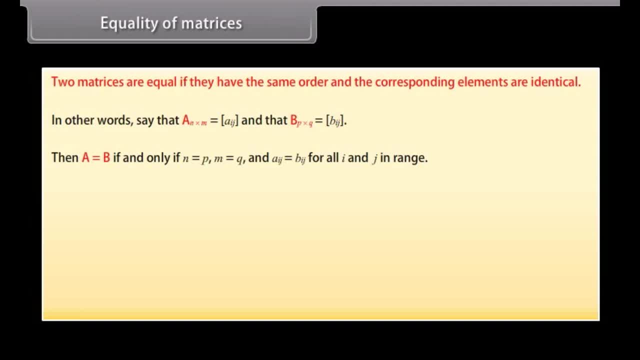 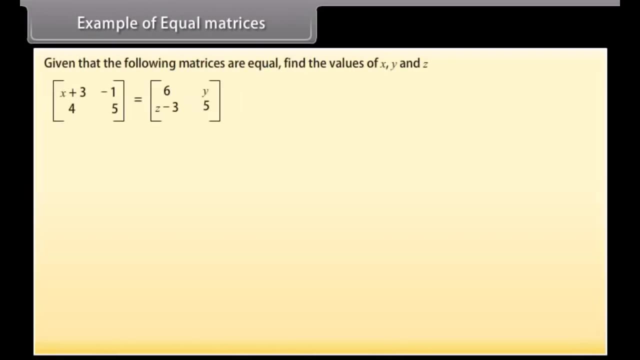 for all i and j in range. Matrices p and q are equal. Here are two matrices which are not equal. even though they are equal, They have the same elements. Example of Equal Matrices. Given that the following matrices are equal, find values of x, y and z. 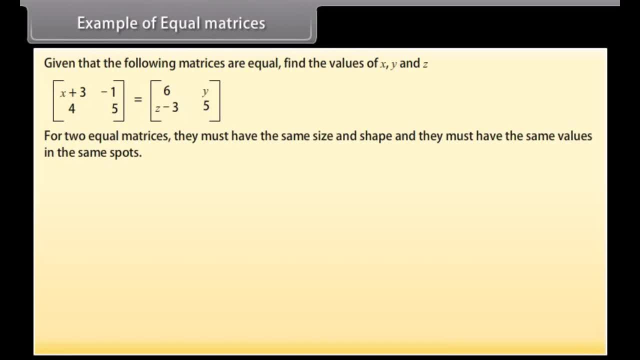 For two equal matrices. they must have the same size and shape and they must have the same values in the same spots. Or we can say: a11 must be equal to b11, a12 must be equal to b11, b12 must be equal to b12. 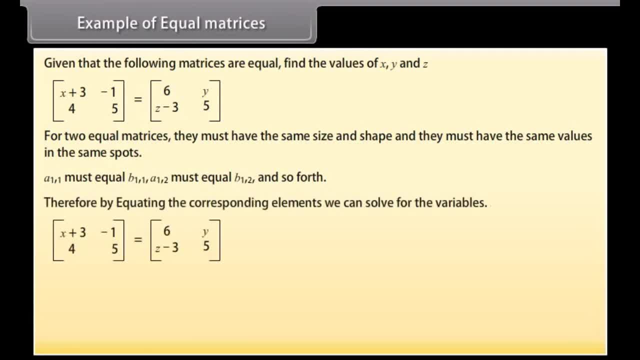 and so forth. Therefore, by equating the corresponding elements, we can solve for the variables: x plus 3 is equal to 6, x is equal to 3, y is equal to minus 1, z minus 3 is equal to 4, z is equal to 7.. 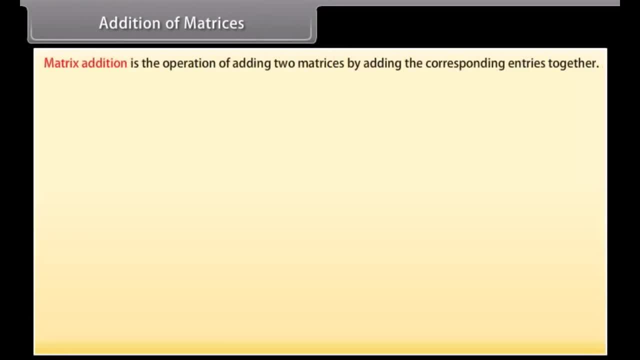 Addition of Matrices. Matrix addition is the operation of adding two matrices by adding the corresponding entries together. Two matrices may be added only if they are of the same order, That is, they must have the same number of rows and columns. Let's add these matrices. 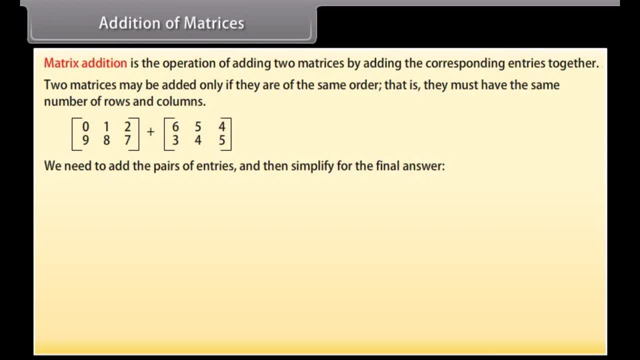 We need to add the pairs of entries and then simplify for the final answer. Row-wise: first row: 0, 1, 2. second row: 9, 8, 7 plus 1. row-wise first row: 6, 5, 4. 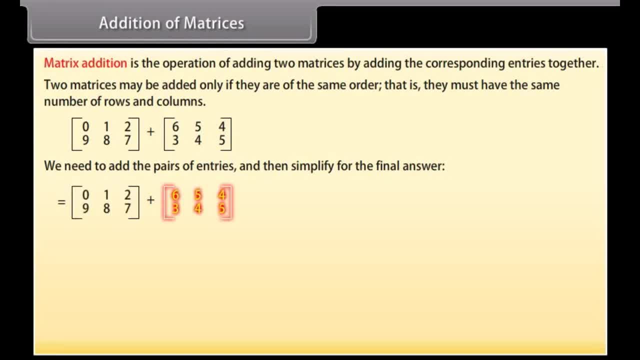 second row: 3,, 4, 5 row-wise. first row: 0 plus 6, 1 plus 5, 2 plus 4. second row: 9 plus 3, 8 plus 4, 7 plus 5 is equal to row-wise. 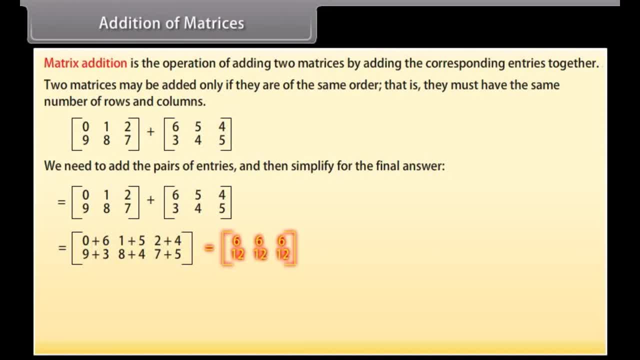 first row 6, 6, 6. second row 12, 12, 12. so the answer is row-wise: first row 6, 6, 6. second row 12, 12, 12. Did you know If A and B are not of the same order? 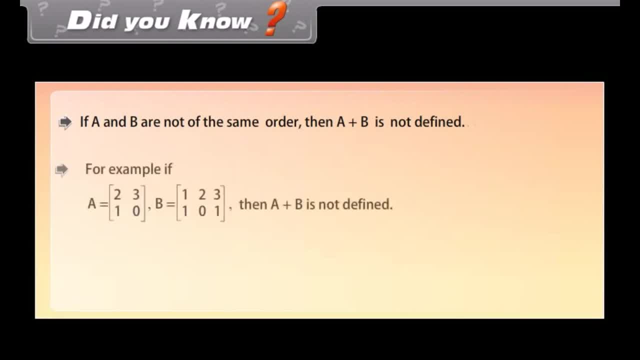 then A plus B is not defined. For example, if A is equal to row-wise first row 2,, 3, second row, 1, 0. B is equal to row-wise first row 1,, 2,, 3, second row 1, 0, 1. 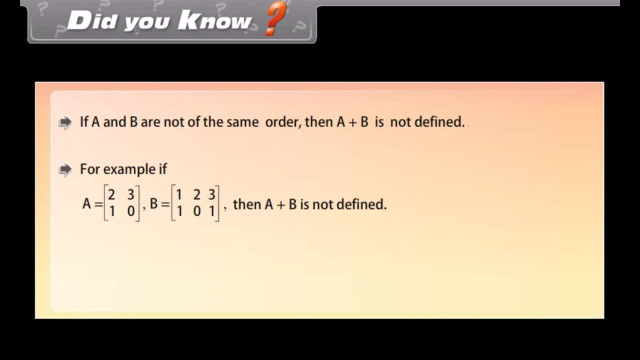 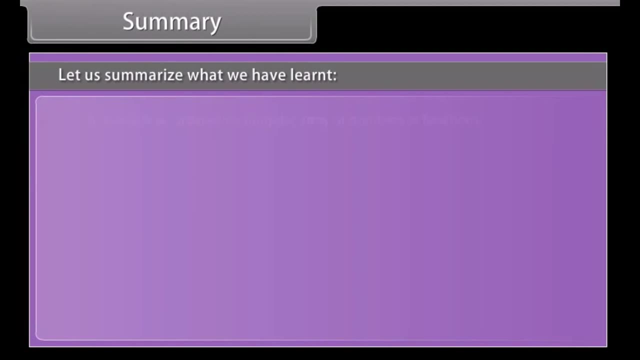 then A plus B is not defined. Addition of matrices is an example of binary operation on the set of matrices of the same order. Summary. Let us summarize what we have learnt. A matrix is an ordered rectangular array of numbers or functions, A matrix having 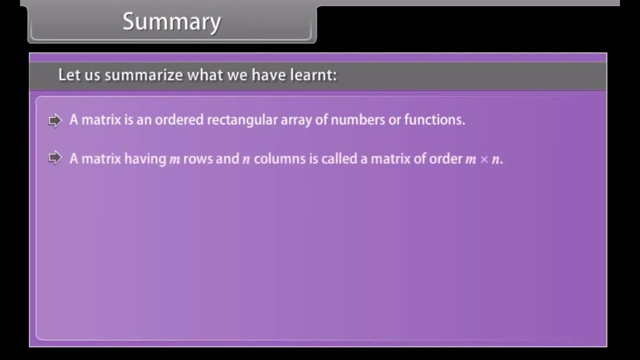 M rows and N columns is called a matrix of order. M by N, A, I, J, M by 1 is a column matrix. A I, J, 1 by N is a row matrix. A N, M by N matrix is a square matrix if M is equal to N. 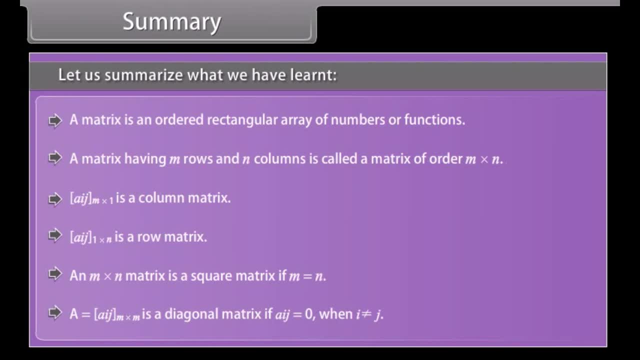 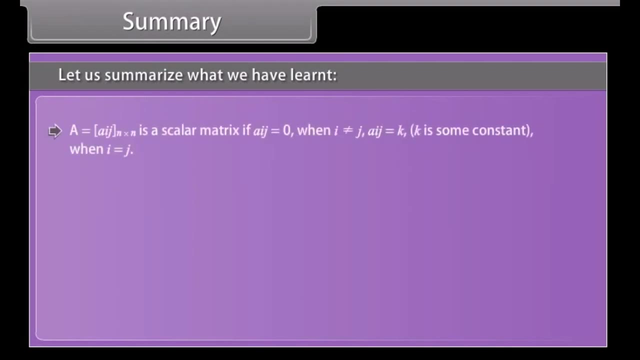 A is equal to A I J. M by M is a diagonal matrix. if A I J is equal to 0, when M is equal to N, A is not equal to J. A is equal to A I J. N by N is a scalar matrix.